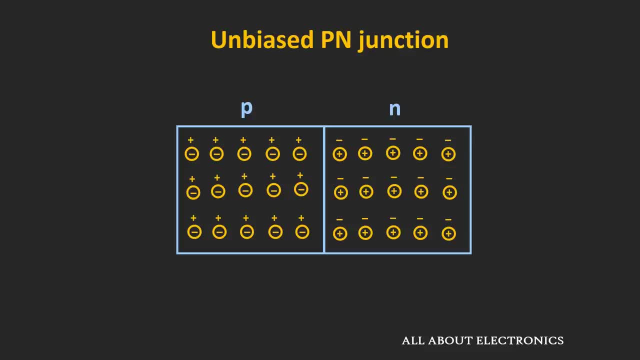 each minus sign represents the electron. And here, for simplicity, in both regions the minority carriers are not shown, But in very small quantity. they are also present in both regions. Now, due to doping, there is a large number of electrons on the n-side, But very few electrons are present on the p-side, Because on the p-side 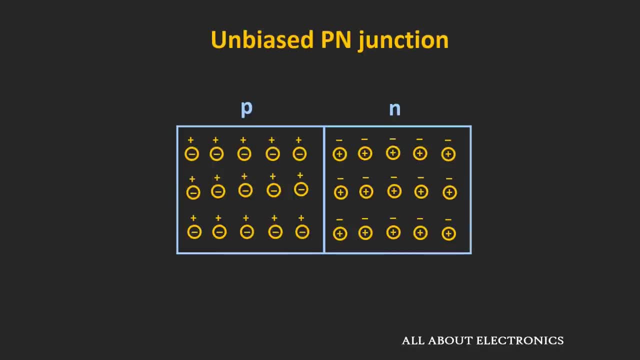 the electrons are minority carriers And whenever this P and N regions are joined, then the electrons from the N side starts diffusing towards the P side. So whenever the electron enters the P-type region, then it becomes the minority carrier And, being surrounded by so many holes, its lifetime will be very short. 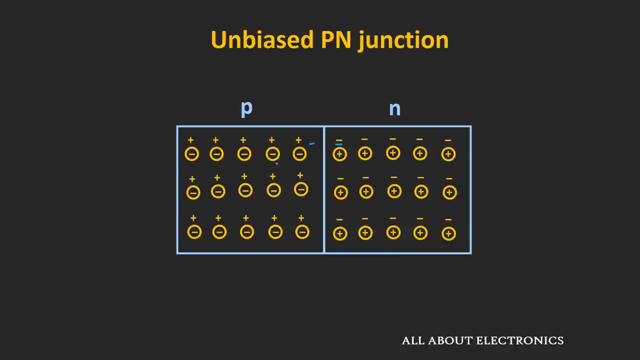 And due to that it will get recombined with these holes. So whenever the electron diffuses across the junction, then it creates the two ions. So first, whenever it leaves this N-type region, then it leaves behind this pentavalent atom. 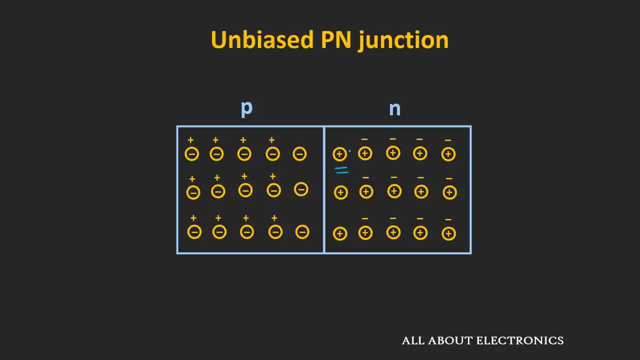 which is just one shot of electron. So due to that it will become a positive ion, And whenever the electron enters this P-type region then it will get recombined with the hole of this trivalent atom. So after capturing the electron, 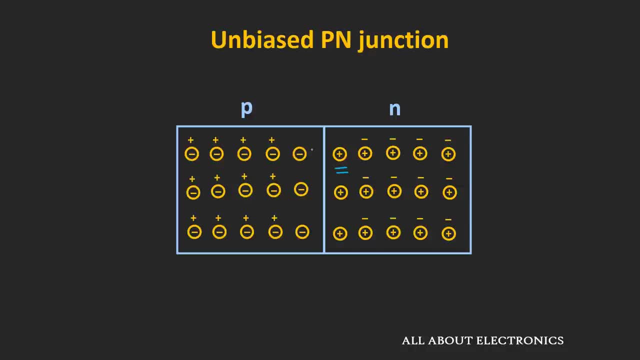 this trivalent atom will become a negative ion. So every time the electron diffuses to the P-side from the N-side, then it creates one positive and the negative ion near the junction. Now these ions are the immovable ions And, unlike the free-charge carriers like electrons and the holes, they cannot move. 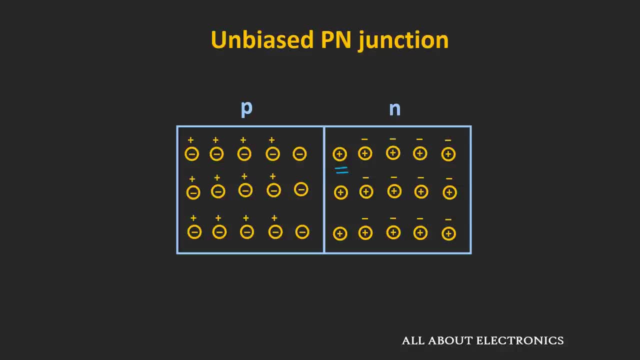 So, due to the recombination of these holes and electrons near this junction, there is hardly any free-charge carriers near this junction. Or we can say there are no free-charge carriers near this junction, Or we can say there are no free-charge carriers near this junction. 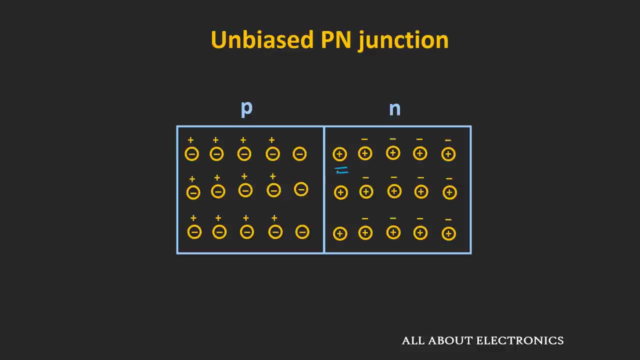 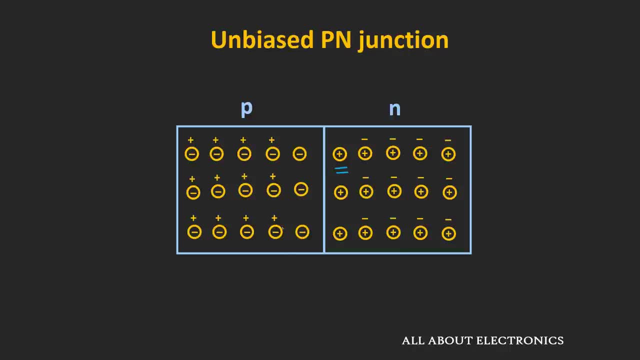 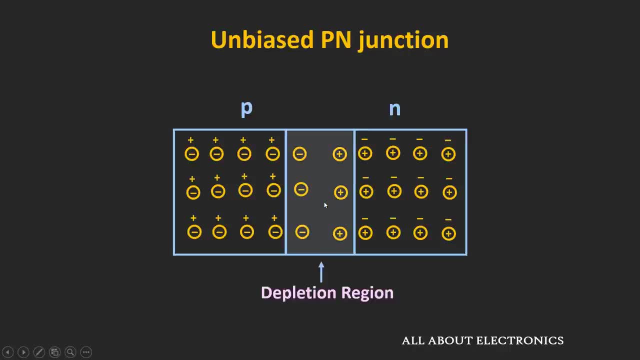 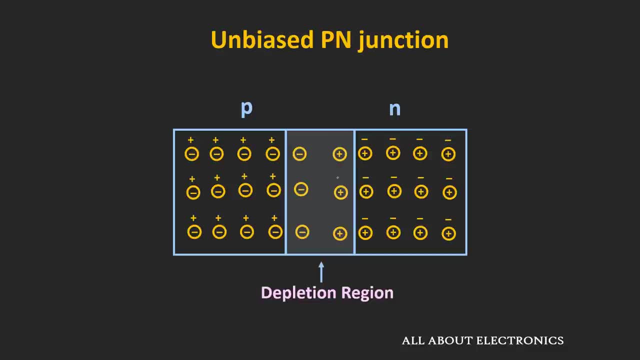 So this depletion region contains both positive and the negative ions which are immobile in the nature, And apart from that, it also contains a few charge carriers which are thermally generated in this depletion region. Now, in this depletion region, these ions sets up the electric field. 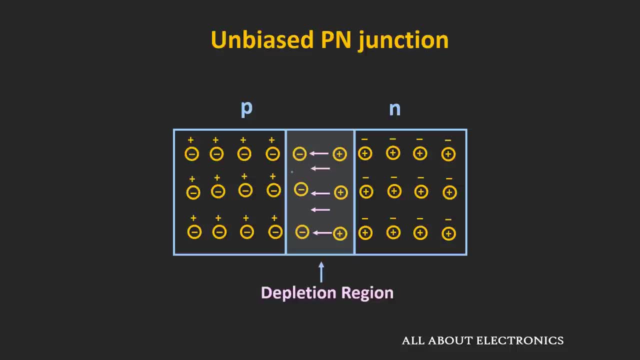 And this electric field points from the positively charged ions towards the negatively charged ions And, due to this electric field, only few electrons are present. electrons from the ion side are able to cross this depletion region, And the same is true for the holes in this P-side region. 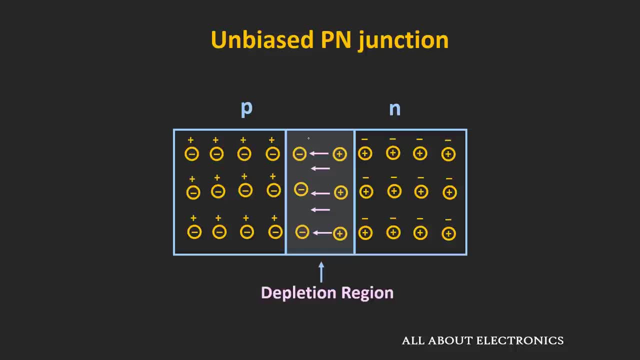 Or we can say that these immobile ions create the barrier potential for these majority carriers, So that they are not able to diffuse from one side to the other side. So this barrier potential is also known as the built-in potential, And for the silicon this built-in potential is equal to 0.7 V. 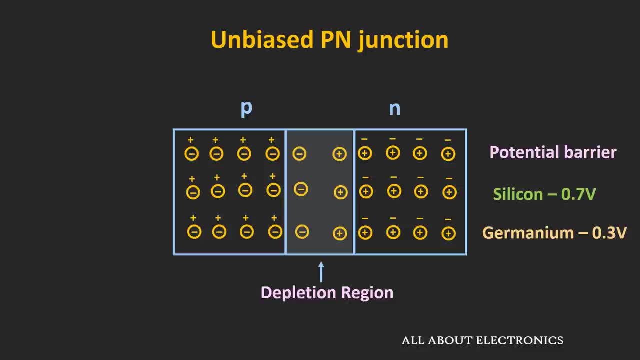 While for the germanium it is roughly around 0.3 V. So the free charge carriers, or, to be precise, the majority carriers in both regions, has to overcome this barrier potential to cross this depletion region, And only few majority carriers are able to cross this barrier whenever there is no external 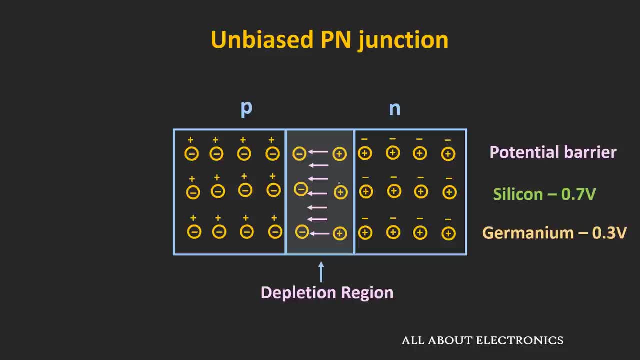 biasing But due to this electric field, the minority carriers in both regions will be able to cross this depletion region. For example, The holes which are minority carriers in this n-type region will get swept from the n-type region towards the p-type region. 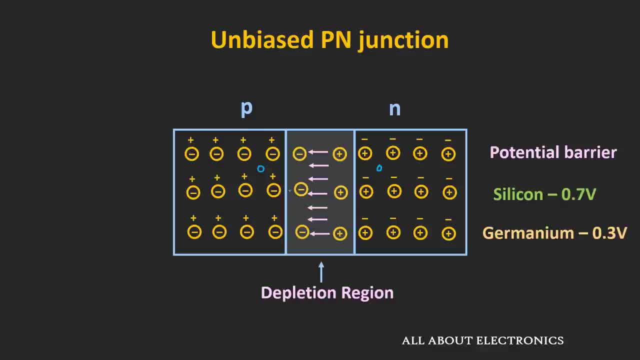 And they will become a majority carriers in this p-type region. Similarly, the electrons, which are minority carriers in this p-type region, will get swept due to this electric field in this n-type region And once they enter this n-type region, they will become the majority carriers. 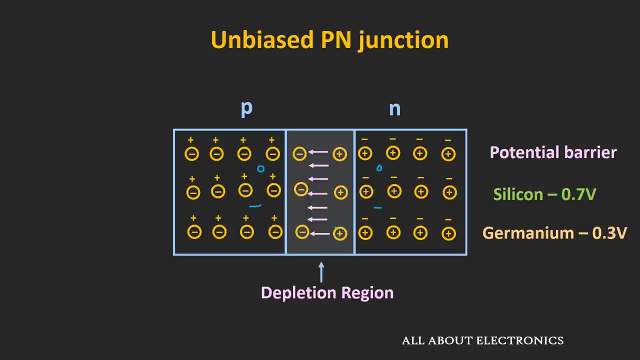 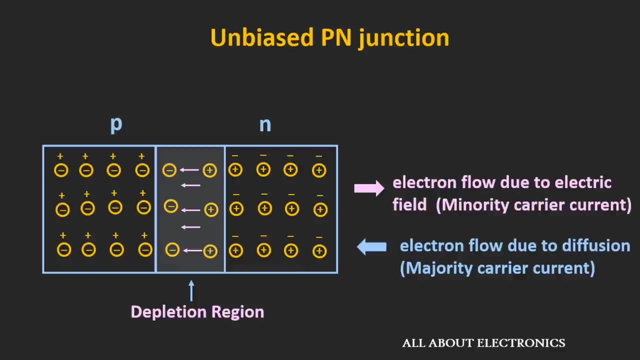 So, due to this built-in electric field, the majority carriers are not able to cross this junction, But still the minority carriers will be able to go from one region to the another region. But when there is no external biasing is applied, then the flow of electrons due to the electric 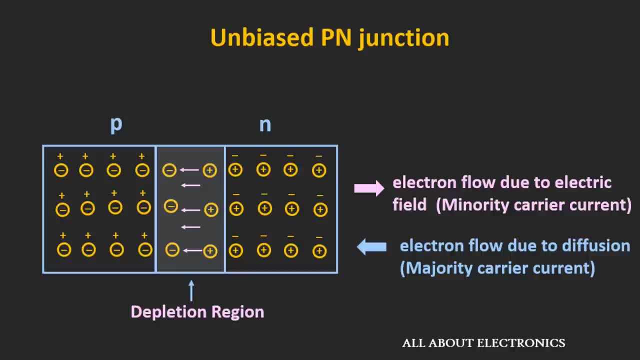 field and, due to the diffusion, will get cancel out each other. Or in other words, we can say that the flow of minority charge carriers and the majority charge carrier will cancel out each other, So that the overall current in the circuit will be zero. 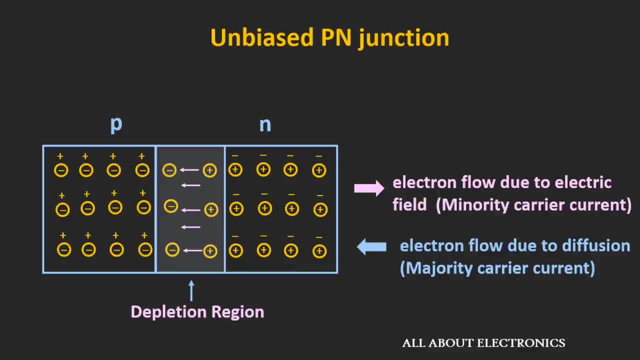 And the same thing is also applicable for the holes. So whenever this p-n junction is not biased, then the overall current in the circuit will be zero. So if these majority charge carriers on both n and p side wants to cross this depletion region, then they require the external biasing voltage. 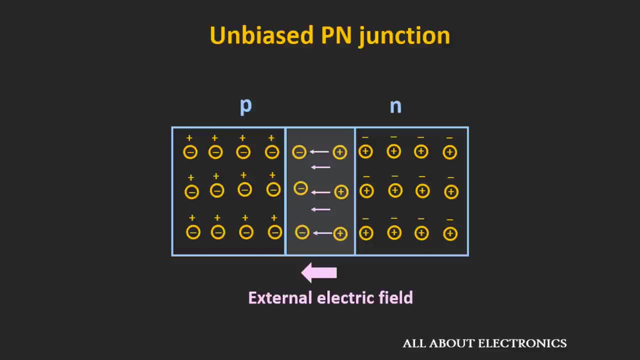 So if we apply the external field in the same direction as the built-in electric field, in that case this depletion region will provide a more resistance to the majority carrier. On the other hand, if the applied external field is in the opposite direction to the 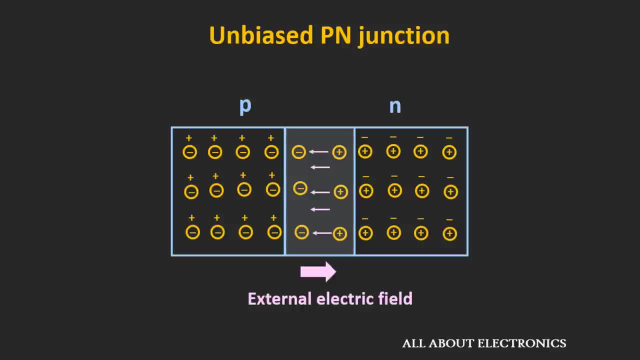 built-in electric field. in that case the resistance which is offered by the depletion region will reduce. So, based on that, let's see the two types of biasing for this p-n junction, And first let's talk about the forward bias- p-n junction. 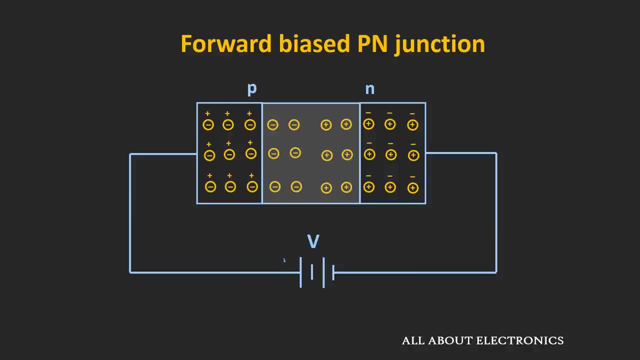 So in case of a forward bias, 1. The negative terminal of the source is connected to the p-side and the negative terminal is connected to the n-side And in this forward bias condition the external electric field is in the opposite direction to the built-in electric field. 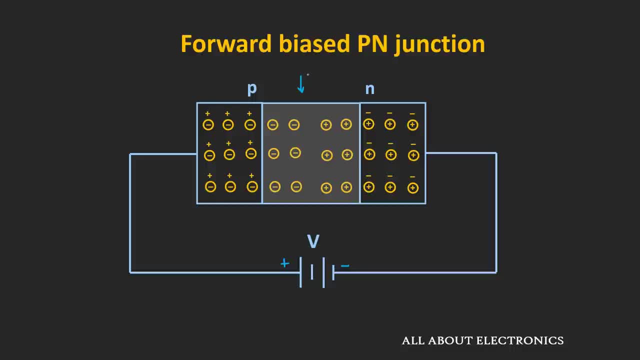 And due to that the effective electric field at the junction will reduce. So in the forward bias condition the electrons in the n-type region and the holes in the p-type region will get pushed towards the junction. So due to that the width of the depletion region will reduce. 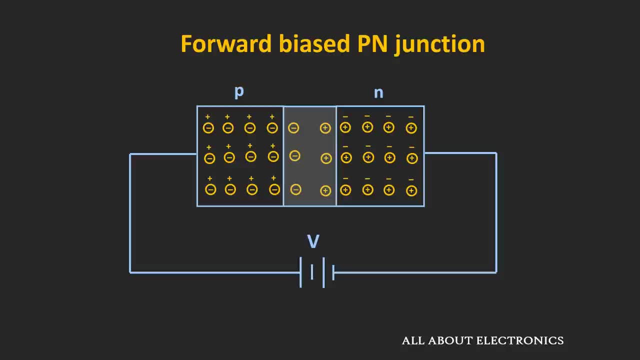 So the effective resistance which is offered by the depletion region will also reduce. So if we further increase the external applied voltage, then the width of the depletion region will further reduce, And when the applied voltage is more than the barrier potential of this p-n junction. 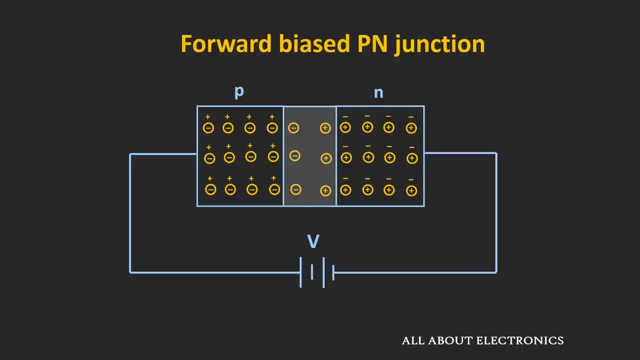 then the resistance that is offered by the depletion region is negligible. So, for example, For the silicon crystal, if the applied external voltage is more than the 0.7V, in that case the resistance that is offered by the depletion region will be negligible. 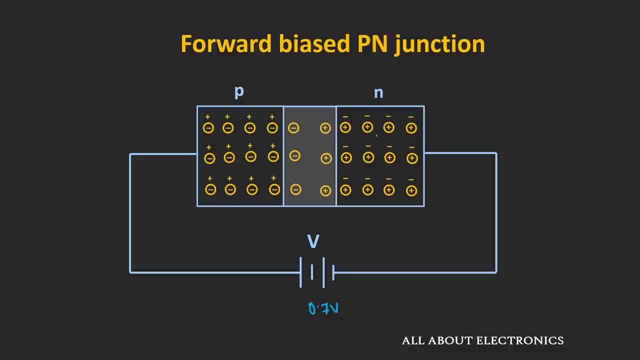 And in this condition the electrons from the n-side can cross this depletion region. And once they cross this depletion region then they will get attracted towards the positive terminal of the battery. So once they come into the p-side region then just by passing through the holes in 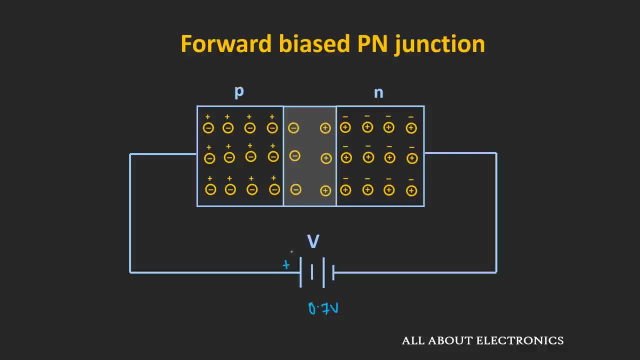 the p-type region, They can reach the positive terminal of the battery And similarly, the holes will be pushed towards the depletion region And once they enter the n-side region, then they will get attracted towards the negative terminal of the battery. So in this way we get a flow of current due to the movement of holes, as well as the electrons. 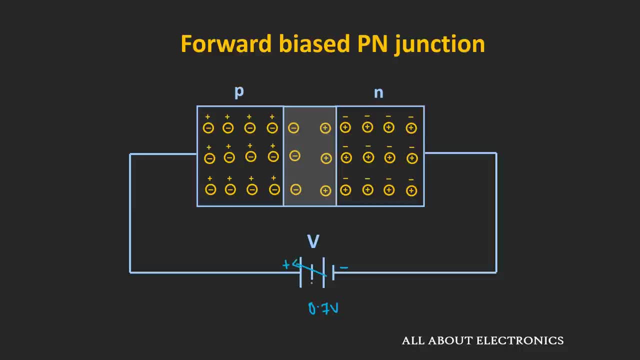 And as we increase the externally applied biasing voltage, the more and more electrons and the holes will be able to cross this depletion region And due to that they will contribute in the flow of current. So as we increase the externally applied voltage, then the flow of current in the circuit will. 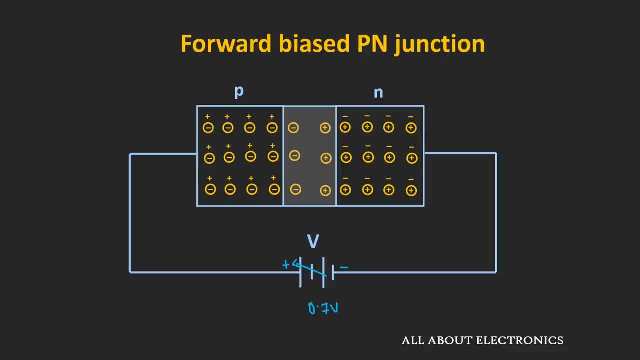 increase. Now, before we go ahead, let me just clear one thing: The hole is nothing but the absence of electron at the particular location. So whenever the electrons are moving from one place to the other place, or here from right to the left, then in a way we can say that the hole is also moving from left to 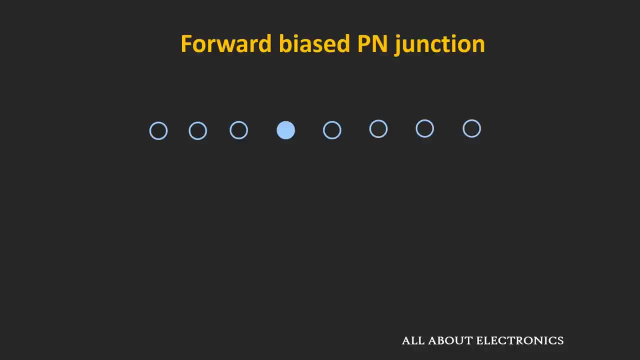 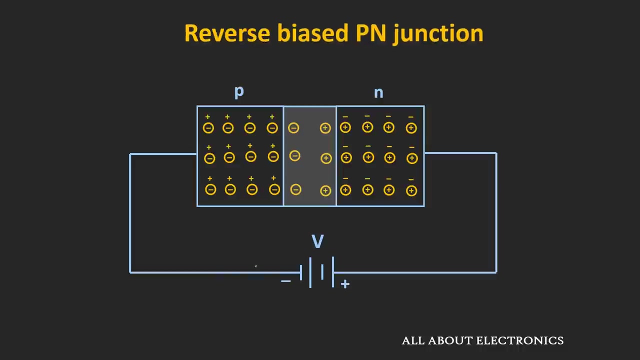 the right. So, due to the movement of electrons, we also get the movement of holes, And in this way we get a flow of current due to the electrons as well as holes. So now, similarly, let's see when the p-n junction is reversed, biased. 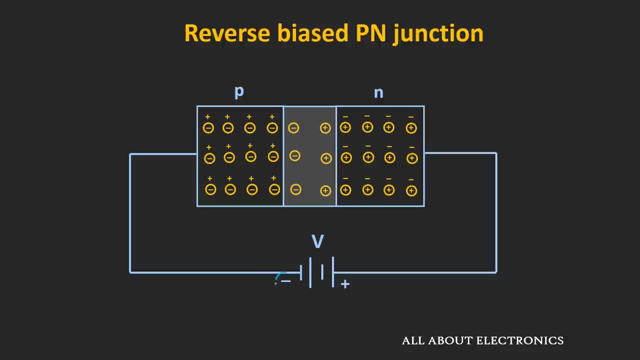 So in the reversed biased condition, the negative terminal of the battery is connected to the p-side And the positive terminal of the battery is connected to the n-side. So in this condition the electrons which are majority carriers in this n-type region will 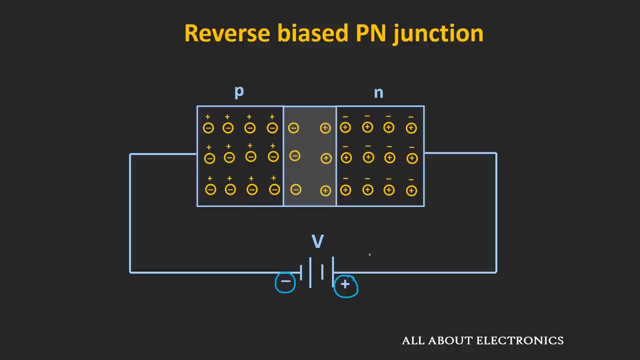 get attracted towards the positive terminal of the battery And similarly, the holes on the p-side region will get attracted towards the negative terminal of this battery And due to that, the more ions will get created near the junction. So we can say that the width of the depletion region will increase. 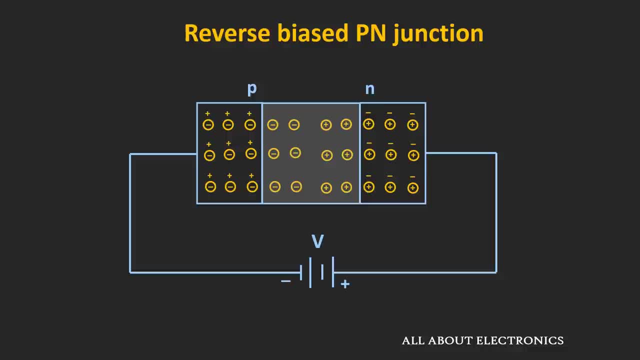 So in the reverse bias condition, as we increase the reverse bias voltage the width of the depletion region will further increase And due to that now this depletion region offers more resistance to these majority carriers And due to that virtually there is no flow of current due to the majority carriers. 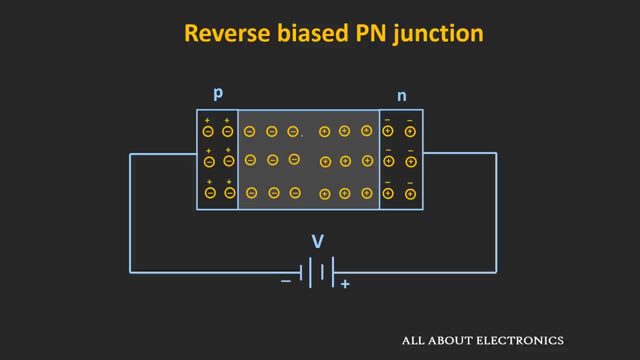 But in this case, due to the built-in electric field, minority carriers in the both regions will be able to cross this depletion region. So in this reverse bias condition, the width of the depletion region will increase. So in this reverse bias condition, the holes which are minority carriers in the n-type 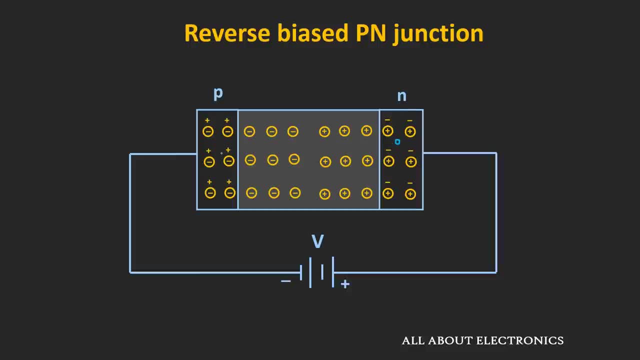 region will cross this barrier and will reach to the p-side region. And once they reach this p-side region, then they will get attracted towards the negative terminal of the battery. Similarly, the electrons in the p-type region, which are minority carriers, will be able to. 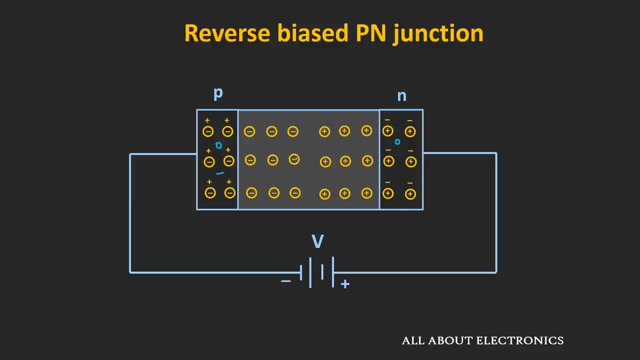 cross this depletion region And after crossing this depletion region they will reach to the n-side region. And once they reach this n-side region, then they will get attracted towards the positive terminal of the battery. So in this way, in this reverse bias condition, we will get a flow of current due to the movement. 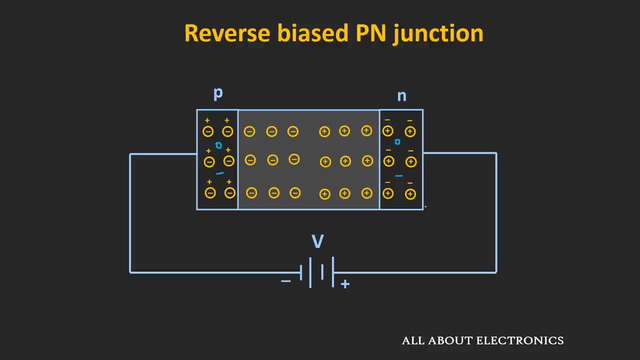 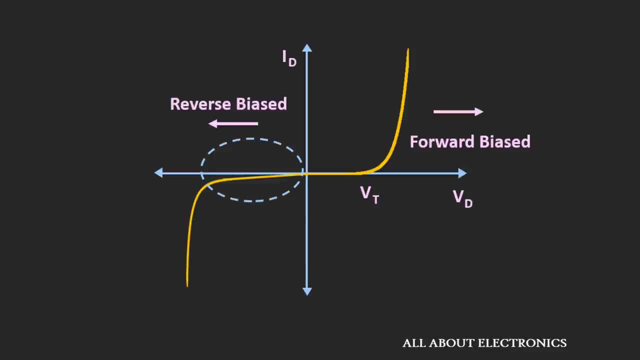 of these minority carriers. But as the minority carriers are very less in comparison to the majority carriers, the magnitude of the current in this reverse bias condition will be very low compared to the forward bias condition. So this flow of current which exists in this reverse bias condition will be very low compared. 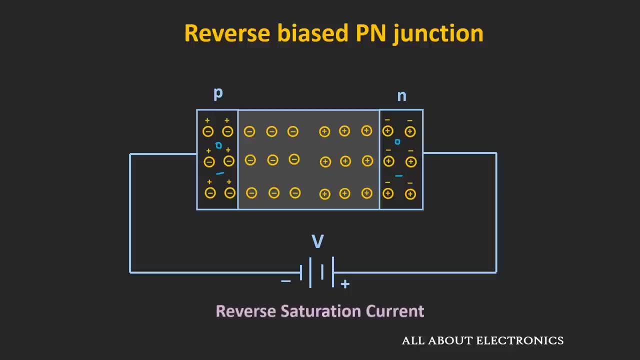 to the forward bias condition. So the current which exists in this reverse bias condition is known as the reverse saturation current, And the term saturation comes from the fact that it reaches the maximum level very quickly and it does not change significantly whenever we increase this reverse bias voltage. 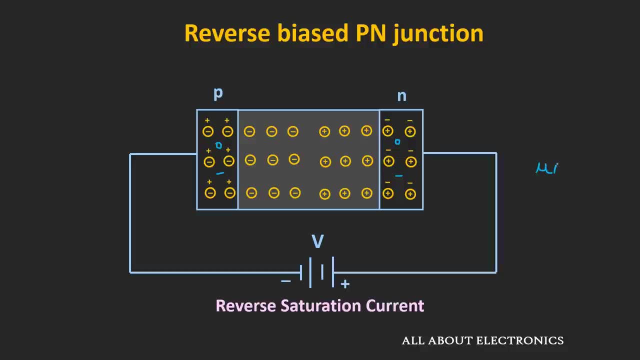 Now, typically, this reverse saturation current used to be the range of micro amperes, But nowadays, due to the advancement in the technology for the silicon devices, this reverse saturation current used to be in the range of micro amperes. So this is the reverse saturation current. 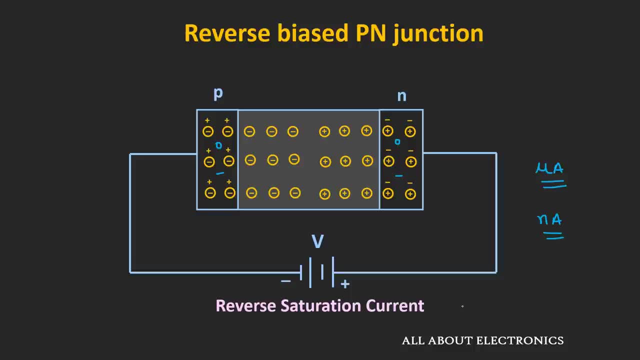 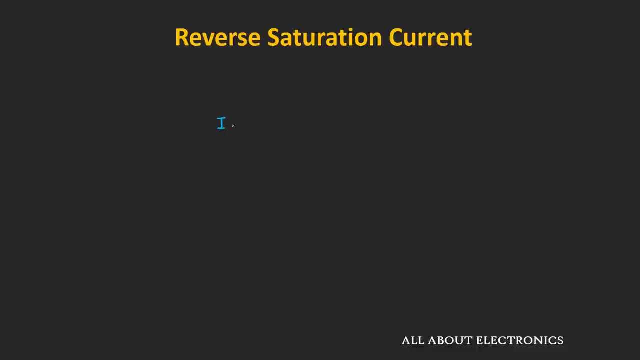 It is a function of the number of nano amperes, And here let's denote this reverse saturation current as Is. So this reverse saturation current is a function of temperature, So as the temperature rises, the thermally generated electron-hole pair in the silicon.